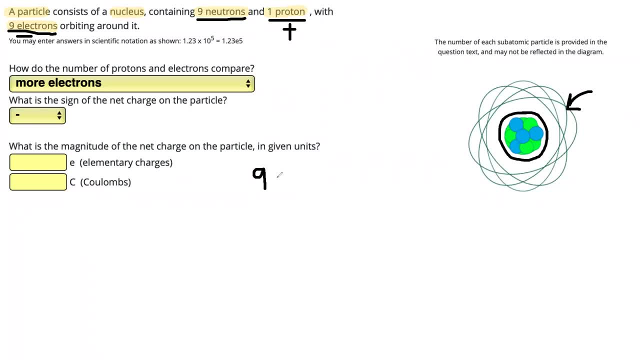 Each electron has a charge of negative e. So we have nine multiplied by negative e Or negative 9e charge for our electrons. Protons have a positive charge. We have one proton with a charge of positive e, So the charge of our proton is just going to be e, So our total charge on our particle is negative 9e. 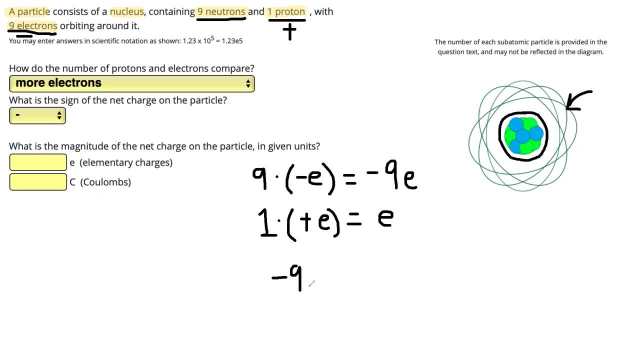 and e. So if we add those together, negative 9e plus e. that gets us a charge of negative 8e. So the net charge we have is to do with how many more of one particle we have compared with the other. And it's negative because we had more electrons than protons. This e. that means 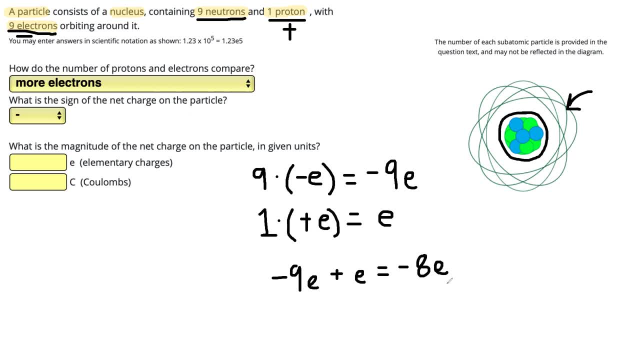 elementary charge, The charge on a proton or a neutron. sorry, the charge on a proton or an electron, It's the same for both, apart from electrons are negative and protons are negative. So we have a negative and protons positive. So our overall charge magnitude: 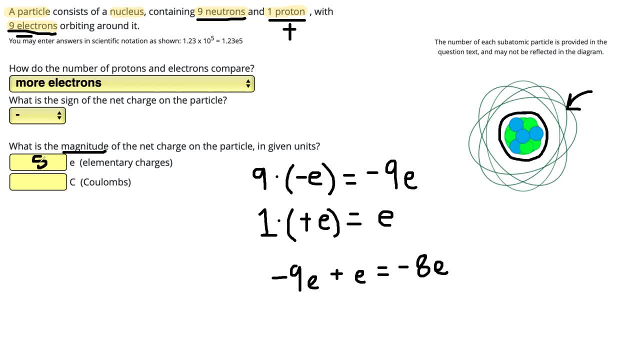 that means we don't need to include the negative is 8e. Final thing we can do is find that in units of coulombs, e is the elementary charge on one proton or one electron And it has a value of 1.6 times 10 to the negative 19 coulombs. So a really. 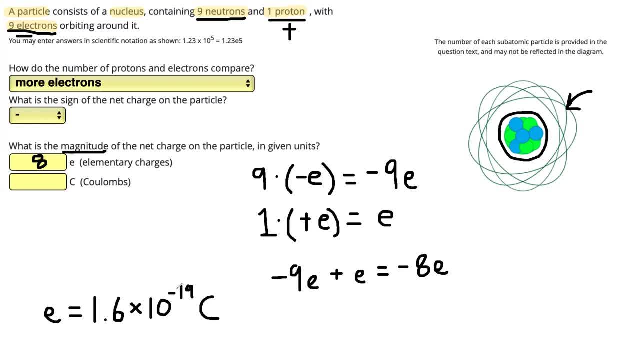 tiny number for the charge on one proton or one electron. So if we know that our charge is 8e, we can calculate that in terms of coulombs by just multiplying out by our e value. So negative 8e is the same as negative 8 times e, which is 1.6 times 10 to the negative 19 coulombs. 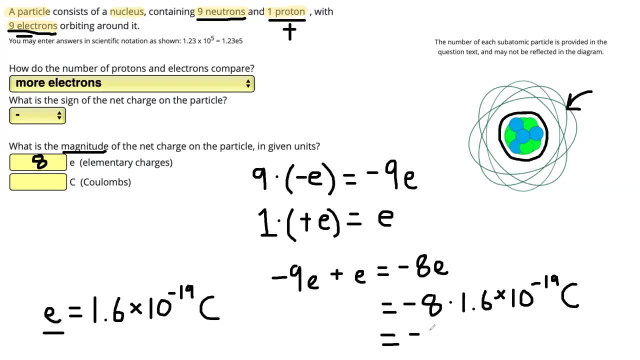 If we multiply that out, we're going to get an answer of negative 1.28 times 10 to the power of negative 18 coulombs. So that's our charge on our particle overall. Again, it asks for the magnitude.